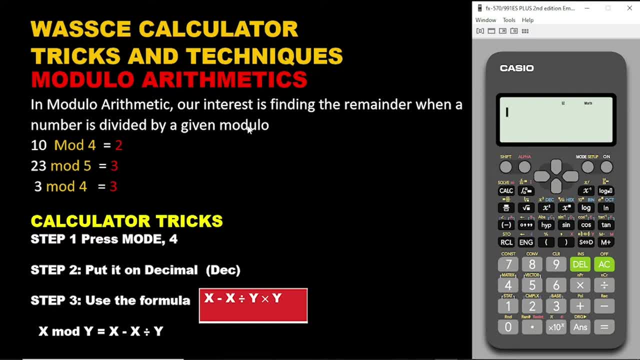 When a number is divided by a given modulo. So, for example, given 10 mod 4 is equal to 2.. This means, when you divide 10 by 4, you will get 2.. Okay, and then again 23 in mod 5, the answer is 3.. That is, when 5 divides 23,, the remainder is going to be 3.. And we can do this so easily. We'll come to the third example. So let's go to the trick. 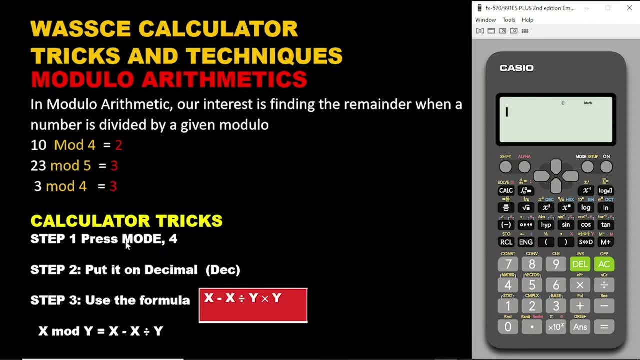 Now the steps that you need to follow is that first you press the mode and then you press the number 4.. So you press the mode and then you pick option 4.. That is number basis. So let's take option 4.. Now, at all times, if you are using your calculator to solve modulo arithmetic, make sure that you see dec- that is, decimal- on the surface of the calculator. Okay, so this is so, so important. 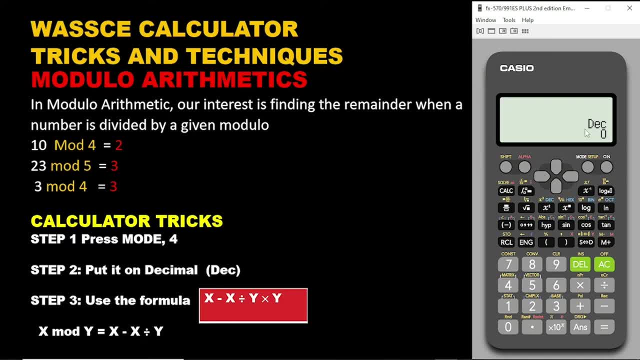 Now let's see To be able to use your calculator to solve modulo in just two seconds. we are going to use this expression: x minus x divided by y times y. Let's explain. So let's say we have this: x mod y. Okay, so x will stand for the number you are going to divide, And then the y will stand for the modulo. So in this example, our x is going to be 10. And then the y is going to be 4.. So 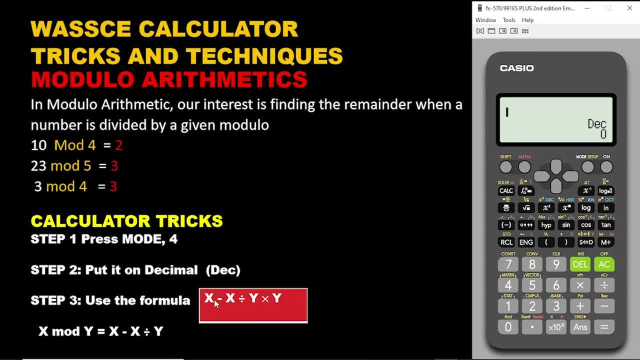 using this simple formula, it's going to be x minus x. So here, if our x is 10,, okay, and the y is 4,, in place of the x we'll put 10 there, And then, in place of the y we are going to put 4 there. So when we use this first example to solve modulo question, it's going to be 10 minus 10, because x is 10.. And then divided by the y is 4.. So divided by 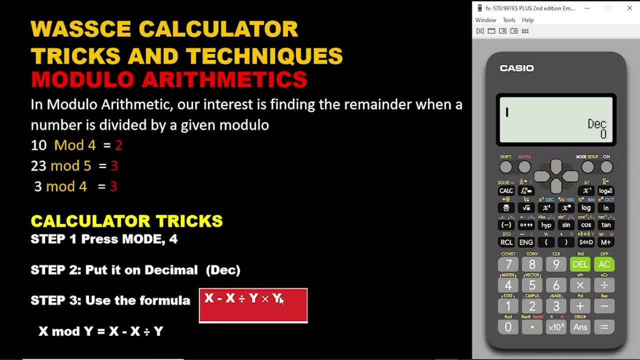 y is 4 times 4.. And that is it. So let's try it and see. So our x is 10.. So we have 10.. Okay, minus 10.. That is x minus x. then divided by, so divided by the y, is the modulo. Okay. so divided by 4 times 4, because we have y times y, Let's see what we get then. further equal sign. Voila, we are there. So. 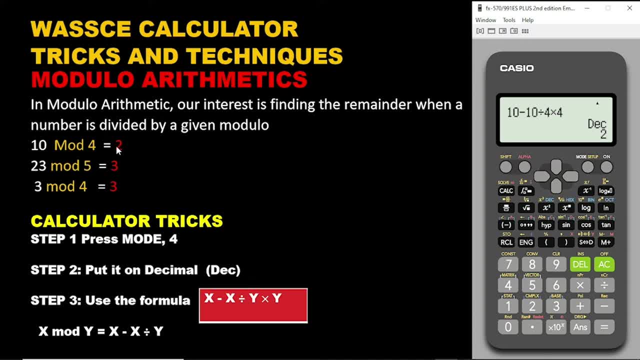 that means this is a simple way of using calculator to solve modulo. Let's do another example: 23 mod 5.. Let's see what we get When 5 divide 23,. what do we get? So, remember, the x is 23.. And then the y is 5.. So we are having 23 minus 23.. Then we divide by y And the 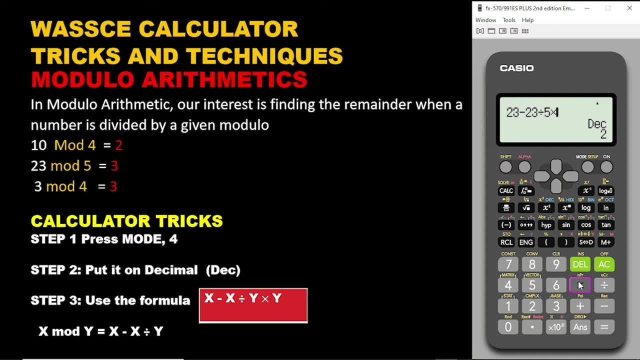 Y is 5.. So that is 5 times 5.. Let's see, Boom, We are there. So that is 3.. Again, let's use the same concept for this. Remember in school you were taught that when the modulo is bigger than the number, 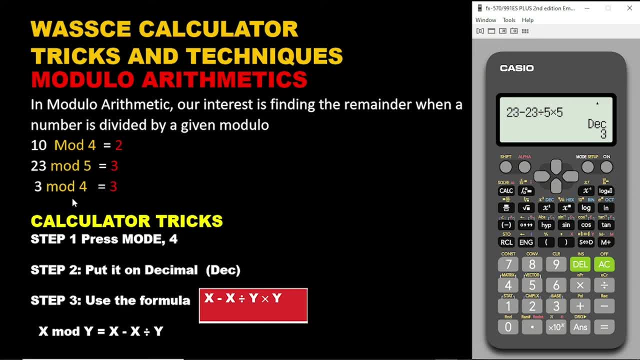 the answer is the number. okay, So here, 4 divided by 4, divided by 3.. Obviously the number is 3 and then the modulo is 4.. So the modulo is bigger than the number. Let's see if we can get the same answer. 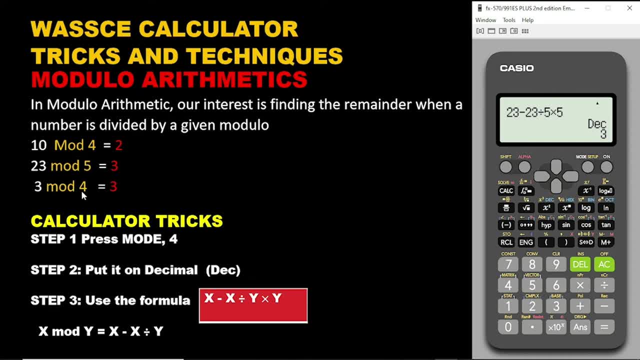 So let's see. So the x is 3 and then the y is 4.. So we have 3 minus 3.. Then you divide that by 4 times 4.. So what do you get? Boom. 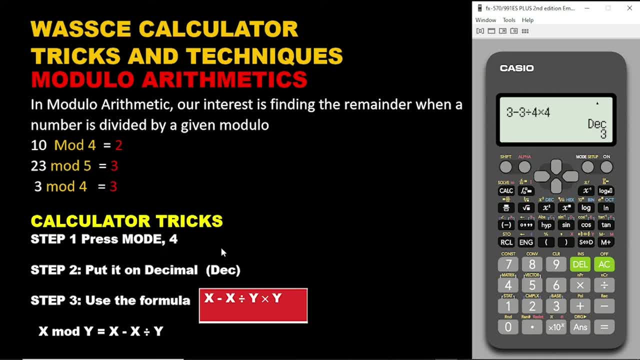 That is 3.. Okay, So what about having a bigger value? Okay, Having a bigger value. Let's say we are dealing with 198. In mod 7. So let's go. So x is 198 and then the y is 7.. 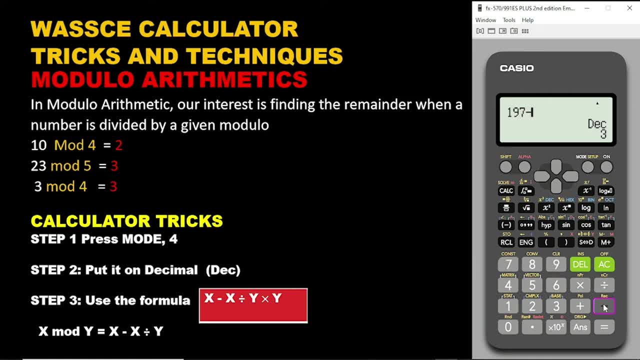 So 198 minus 198. So have it there. Then divide it by y is 7.. So 7 times 7.. What do we get? That is 1.. Okay, So when 7 divides 198, the remainder is going to be 1..